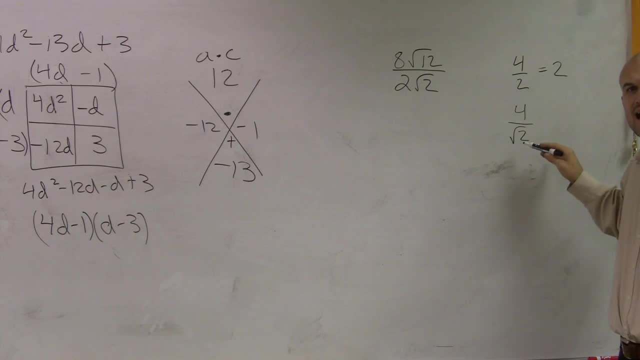 So this is what we call an irrational number. We cannot divide by an irrational number, So therefore we do not want to have an irrational number on the bottom of a fraction. okay, We need to get this radical 2 off there. So what we can do is, if I multiply by a radical 2, well, 2 times radical 2 gives me radical 2 squared right. 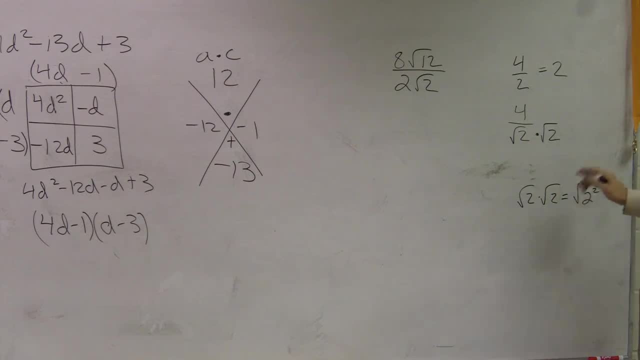 That's 2 times 2, which is 2 squared and the radical 2.. But remember, we're dealing with the square root, So the square root of something squared. those are opposite, They're opposite functions of each other. so we're just going to be left with 2.. 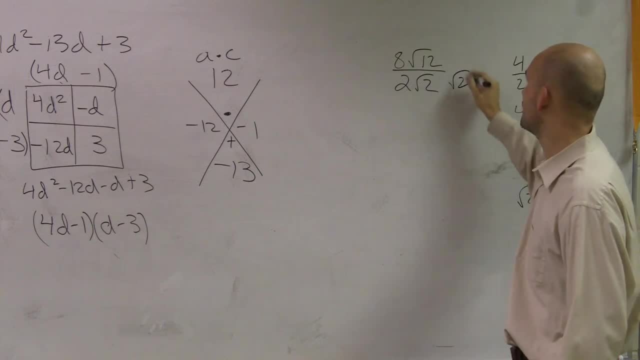 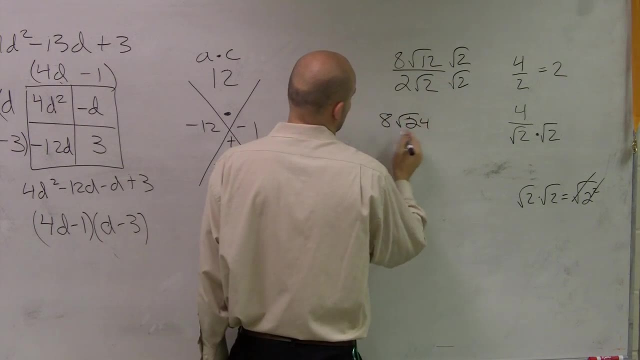 So, on this problem, I'm going to get rid of this radical 2.. So I multiply by radical 2 over radical 2. What I obtain is 8 radical 24. all over 2 times 2 times 2 times radical 2 times radical 2 is radical 2 squared, which is 2.. 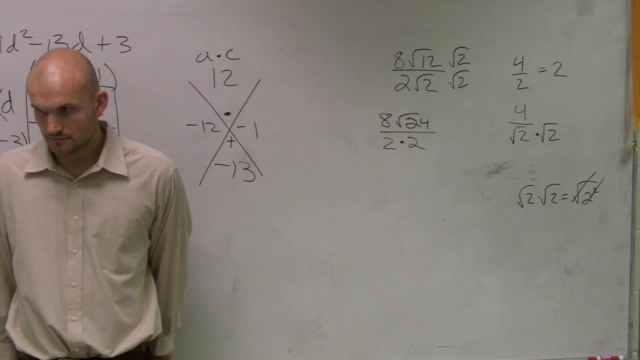 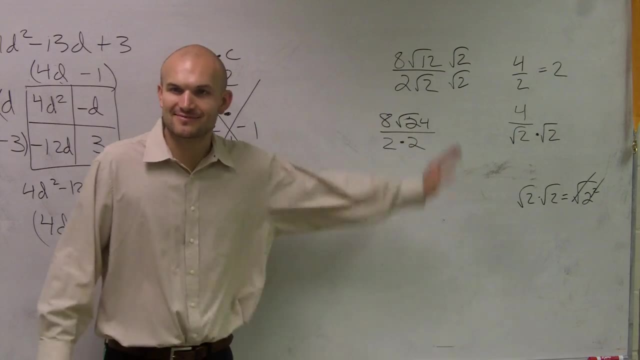 All right, Yep, The radical 2 is supposed to be 3.. Yeah, it's supposed to be 3.. Oh Well, I already have this problem, so we're just going to have to go with this one. but you guys will check with that. 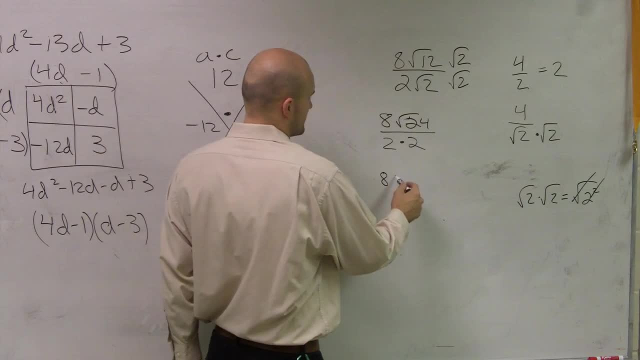 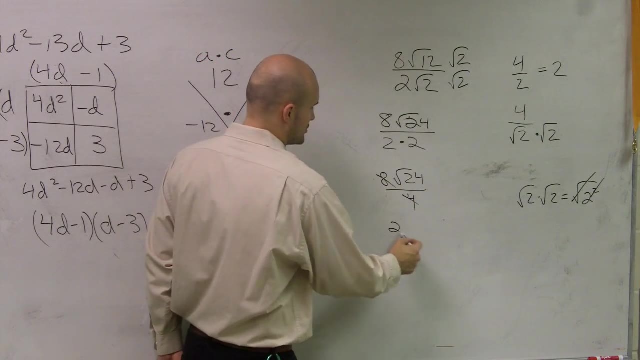 So for this one, if I wanted to do it, I'd have 8 radical 24 over 4, right, Which we know now we can cancel that out to be 2 radical 24.. And then I could say: how can I rewrite radical 24?? 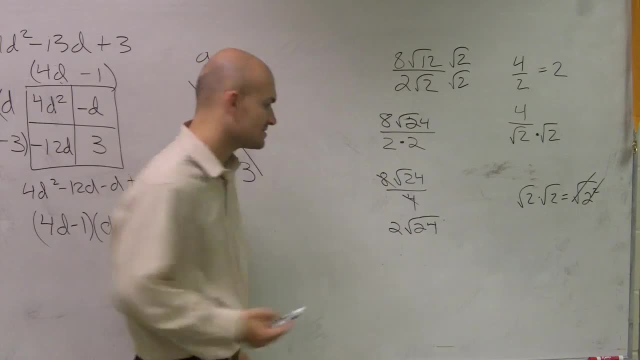 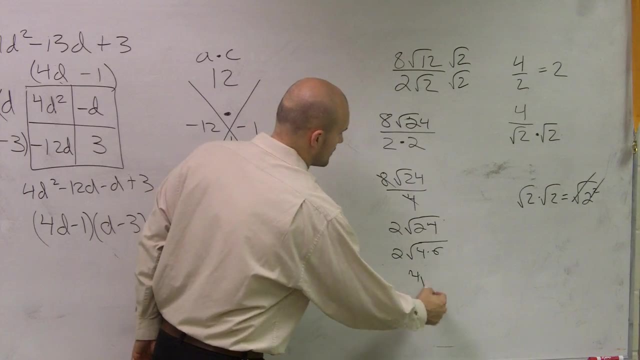 Well, you can rewrite radical 24 as the square root of 4 times 6, right? Which square root of 4 is 2?? 2 times 2 is 4.. Radical 6.. Yeah, it's just breaking it down simple by simple. 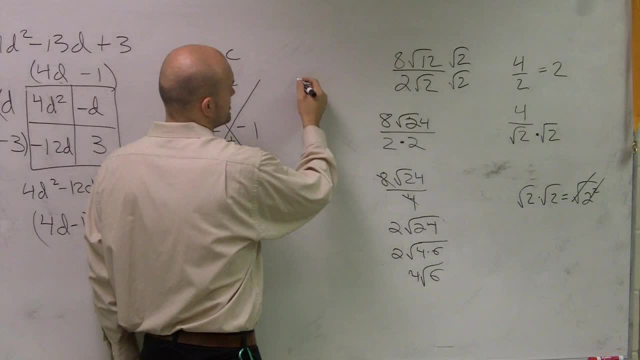 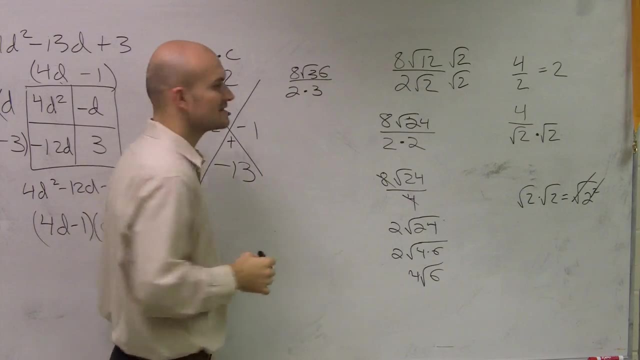 Oh, you guys want radical 3, right, So you multiply by radical 3.. So the 8 radical 36 over 2 times 3.. Well, 8 radical 6 is 6.. 8 times 6 is going to be 48.. 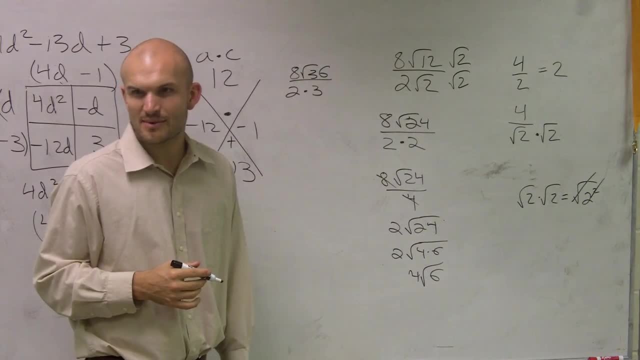 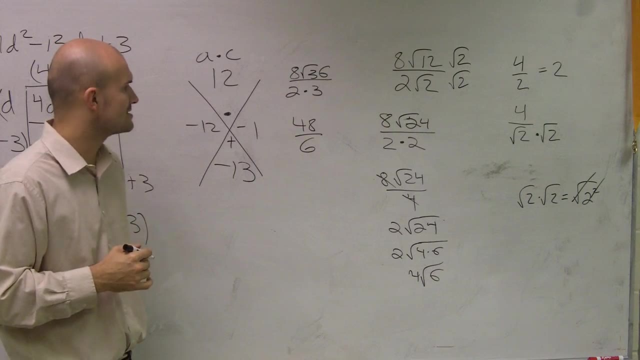 8 times 6,. 8 times 6, right? 48?? 8 times 6, I might lose my mind. 8 times 8 is 48.. Yeah, wow, All right. And then we need to look at that and say: 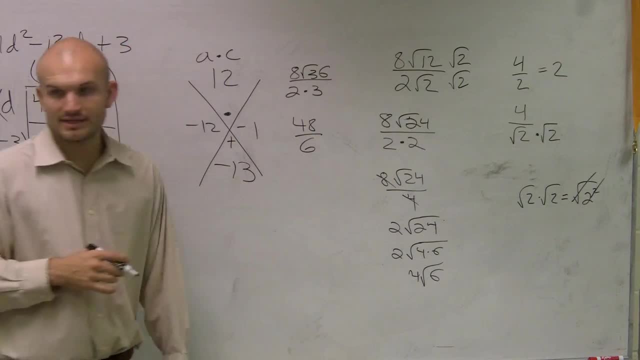 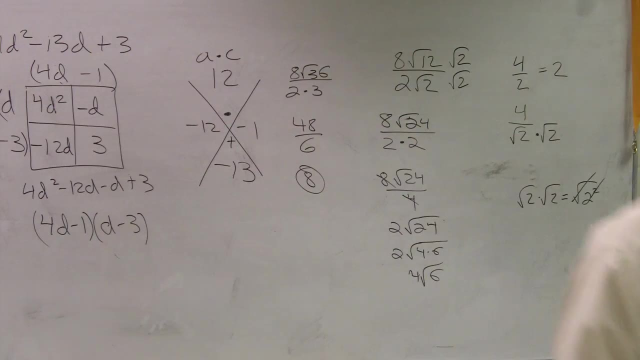 how many times would we break each one of them down? And 48 divides by 6,, 8 times, So that one's a lot easier when you actually have the right problem there, right? Okay, So that's that answer.